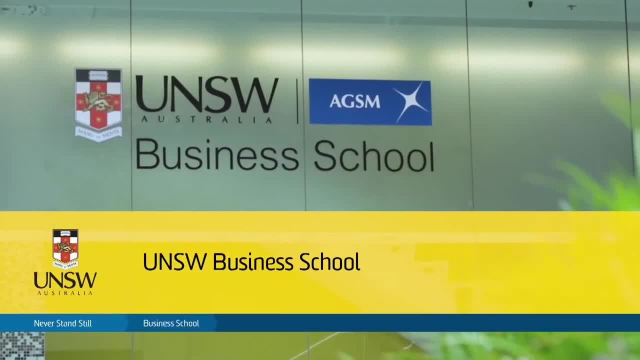 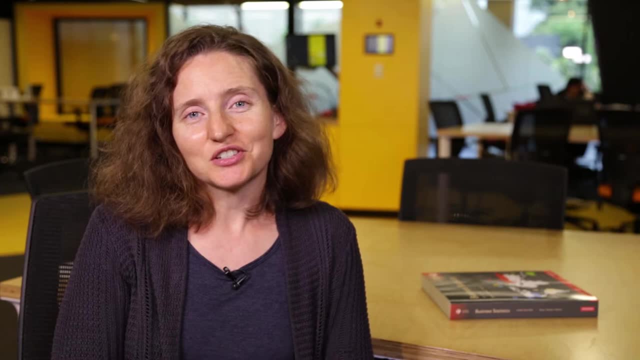 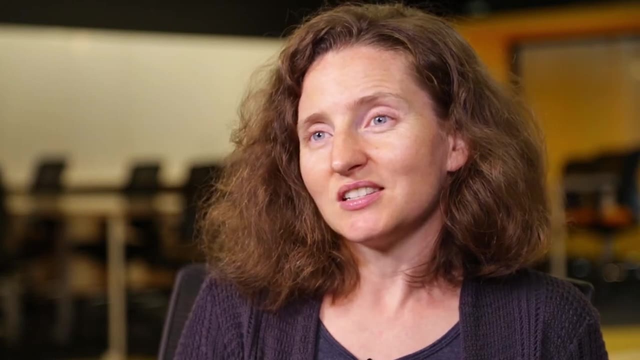 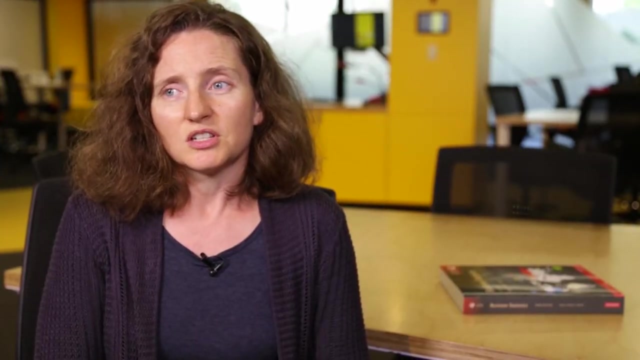 So my name is Gigi Foster and I'm an associate professor in the School of Economics at UNSW Business School. I teach the introductory statistics course, Econ 1203,- Business and Economic Statistics. So the course is the first course that university students here. 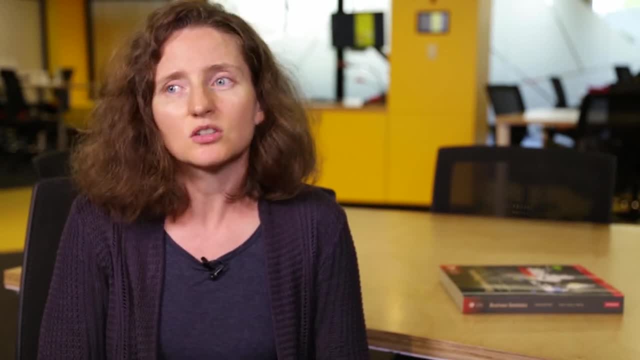 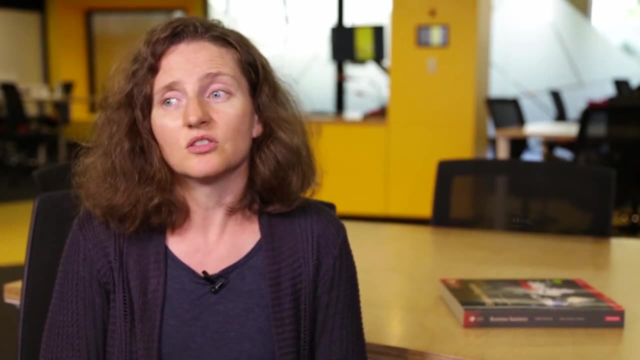 in the BCom and the BX, degrees will take in the statistics or data analysis, And this is important because it's really the only core course whose main focus is on data and the use of data, the interpretation of data for business purposes. And, if you don't know, 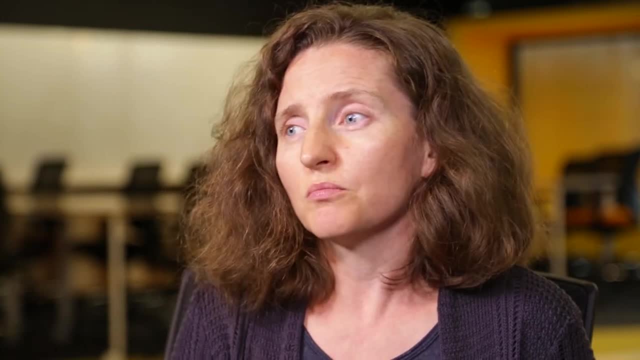 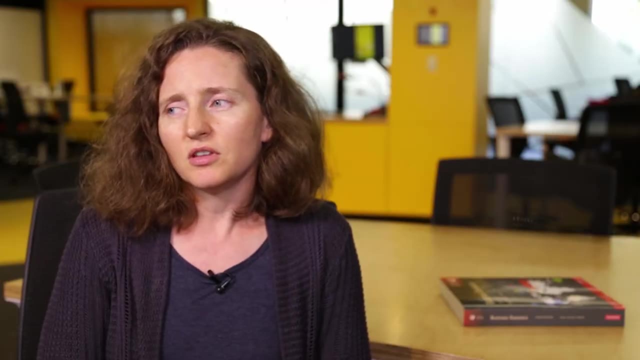 how to do that. then you are hamstrung at a certain point when analyzing a problem. Some problems you can analyze without data. You can just talk about them. You can find solutions. But I find often that when you use data competently, it allows you to think. 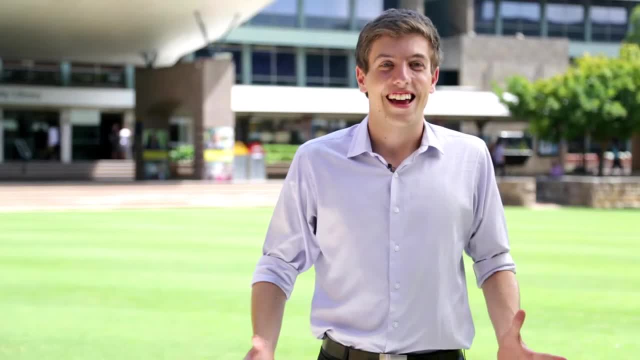 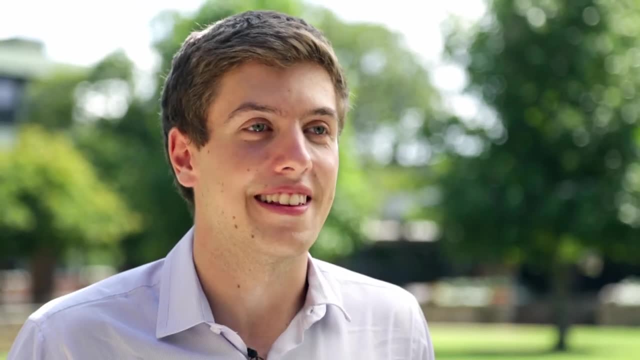 more clearly about a given problem and about its potential solutions. Hey guys, I'm George. I'm a third-year student majoring in finance, and welcome to UNSW. So right now I'm in my third year doing a lot of finance subjects, But in addition, 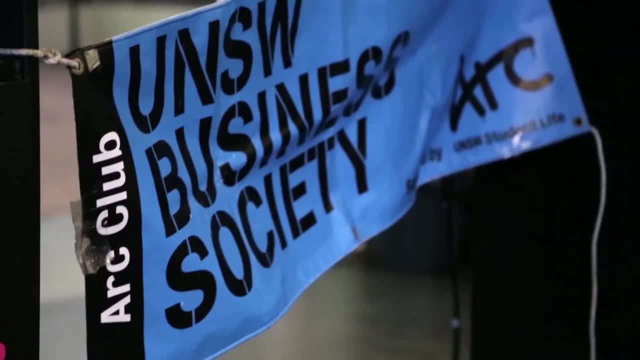 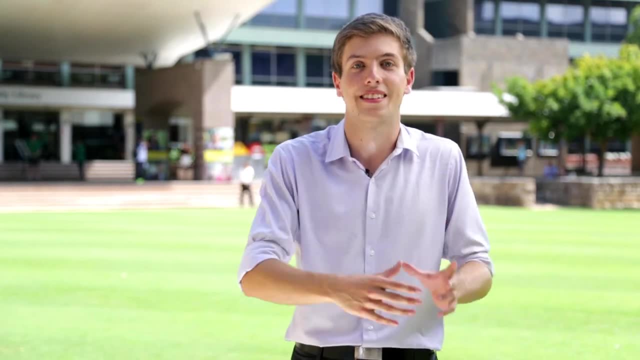 to that. I also do lots of consulting competitions and I'm also part of the business society, And what stats really helped me to do was gain an understanding of how different statistical elements really interplay in the big picture, whether that's finance in sport or just. 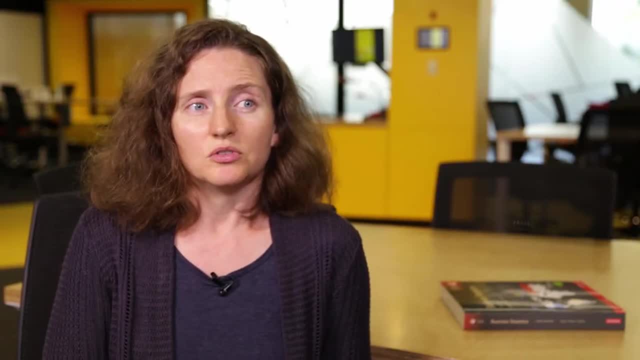 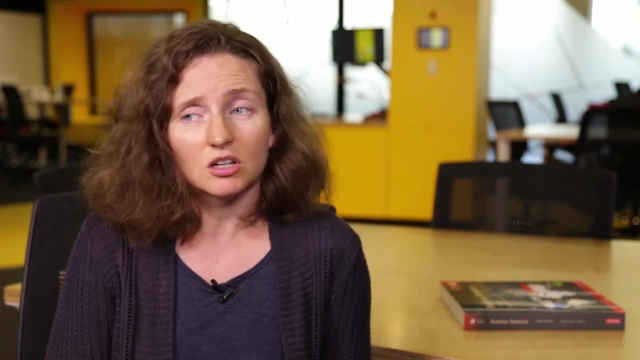 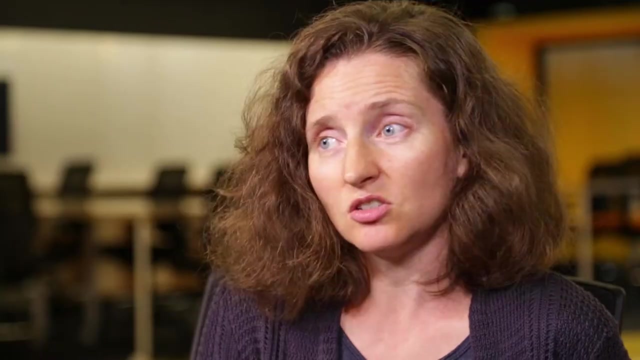 in real life. So people who are numerate and can use data and statistical analyses competently are valued in the world In all sorts of places: in the economy, in the private sector, in companies, consulting firms, in banks, the financial sector. also in the public sector, government departments. 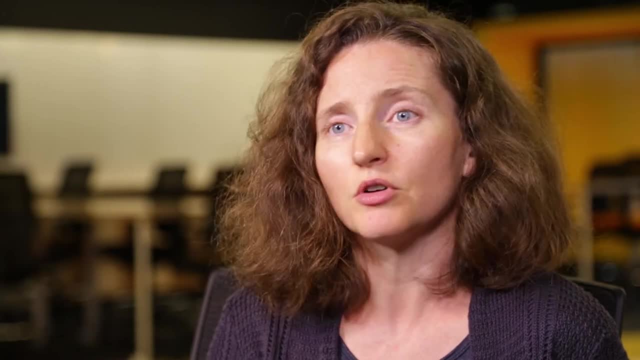 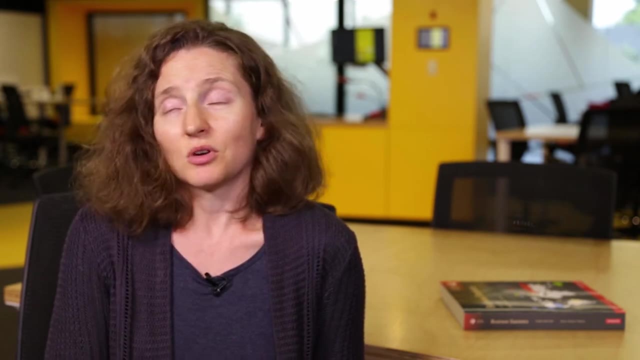 and going into business for yourself, you need to have a head for numbers, So it's a skill set that is widely applicable across a wide variety of different jobs. So I'm very confident. It's one of the reasons I love teaching it, because I want to equip. 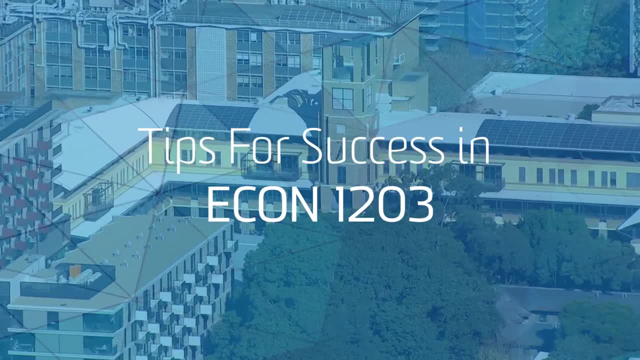 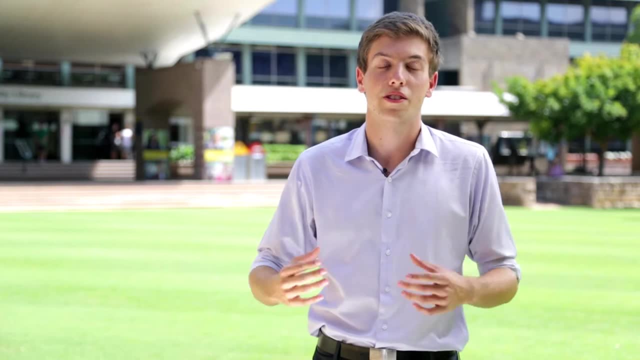 students with that really valuable skill. I guess my biggest tip would be to realize that every concept builds on the previous concept, so it's really important to make sure you understand everything from the start. So if there's something you don't understand, feel free to ask your lecturer or your tutor. 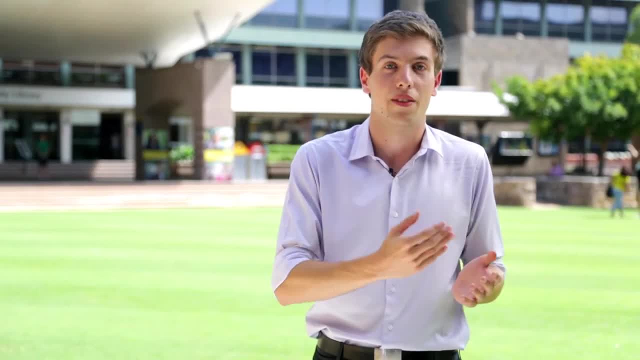 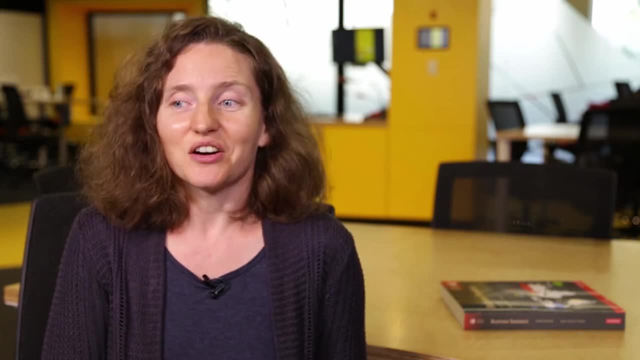 or go to past classes or ask your friends, But just really make sure you understand things from the very beginning, otherwise you'll be in big trouble later on. To do well in this course you basically have to work. You have to do the things that are. 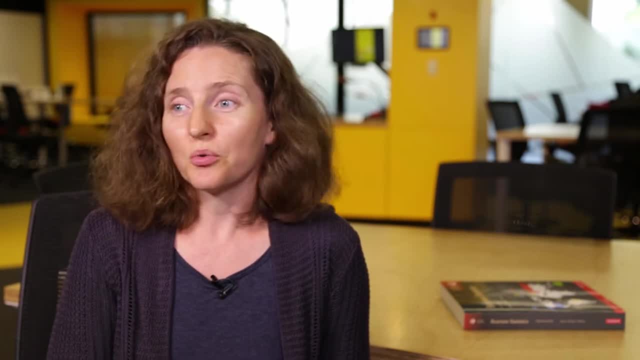 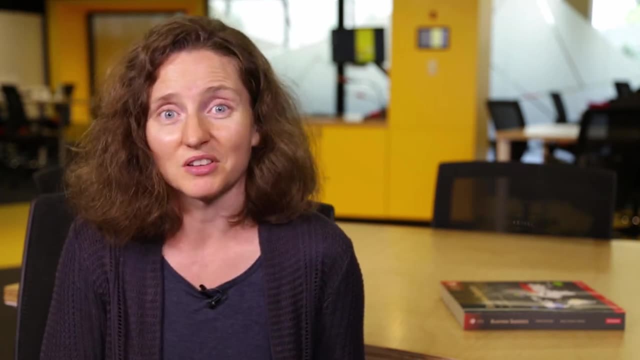 encouraged in the course outline and in your lectures. So we assign readings: do them. We have lectures- come to them, So that's really important. We have tutorial workshops: come to them. We have online resources and quizzes: do them. 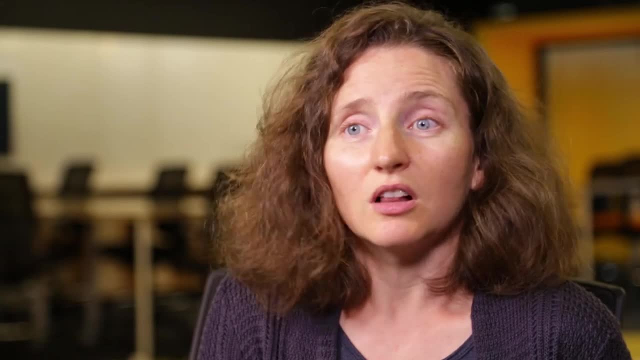 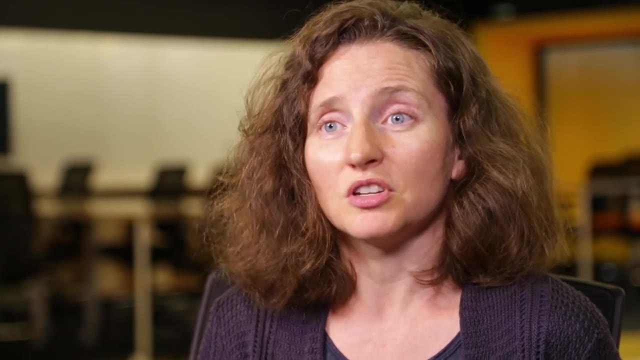 Prepare study. These are the best ways to do well in the course. The students I see failing the course are almost uniformly those students who do not grasp with both hands all the opportunities and all the resources that we provide, and that's a recipe for failure. 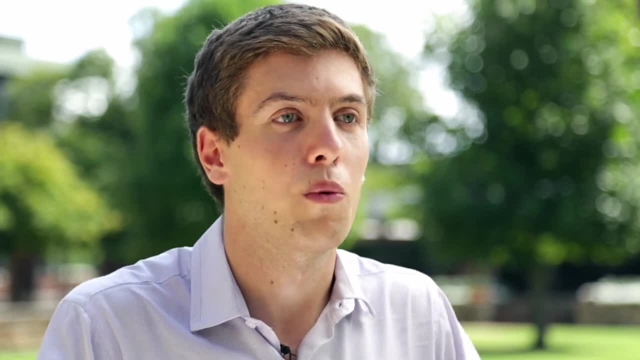 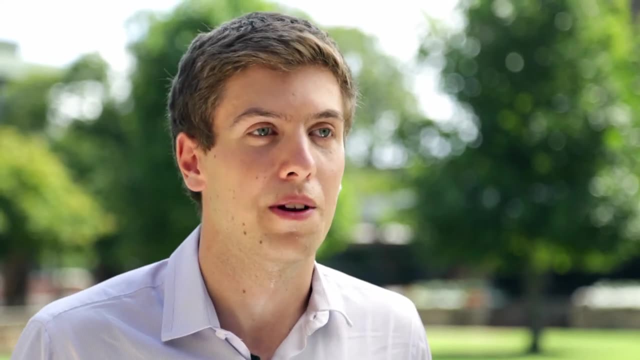 The biggest difference I found with high school was that at high school, everyone always told me what to do, when to do it, by kept giving me constant reminders, whereas at university you're basically on your own And you have to manage your time and manage all your responsibilities, otherwise you won't. 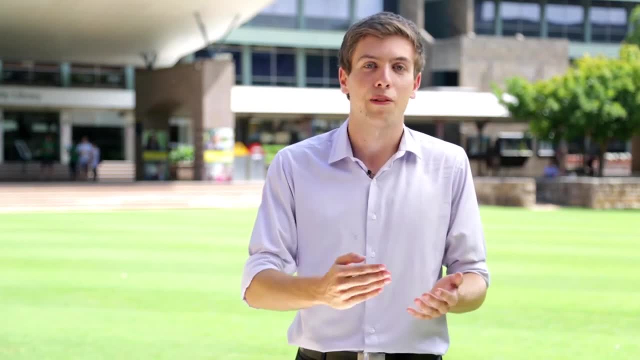 get everything done, And the best way I found to manage this was just to get a plan and really plan out your week, what you have to do and when you have to do it by, and that'll make everything so much easier for you. 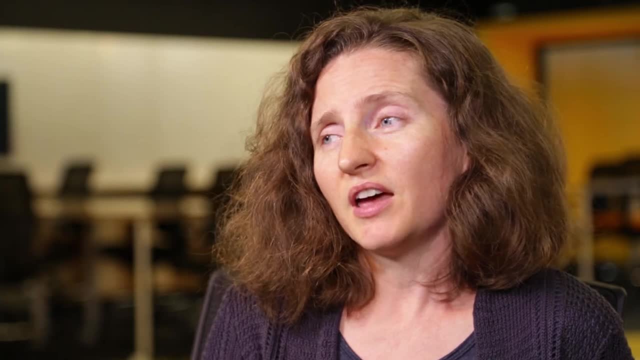 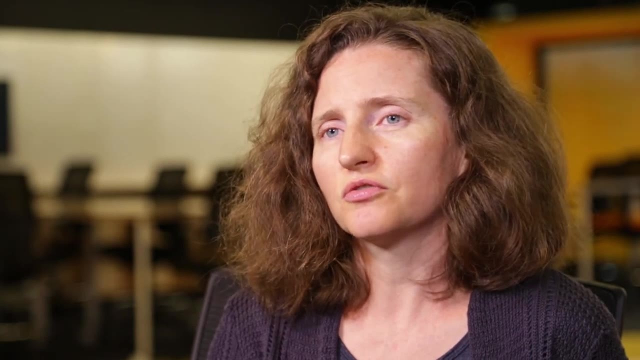 A lot of the people who take this course are taking it because it is the core and they may not really be sure of what they want to do as their next step. So one of the things I advise students regularly to do is use your first year to experiment a bit. Take a course. 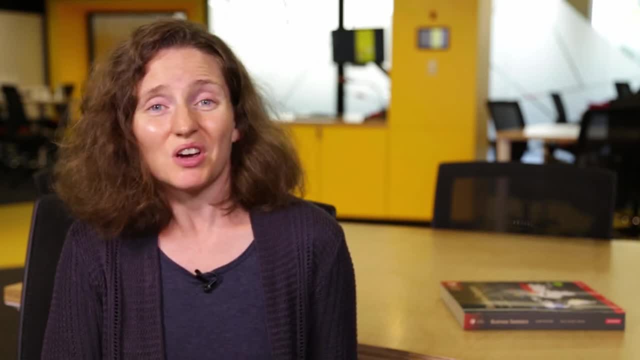 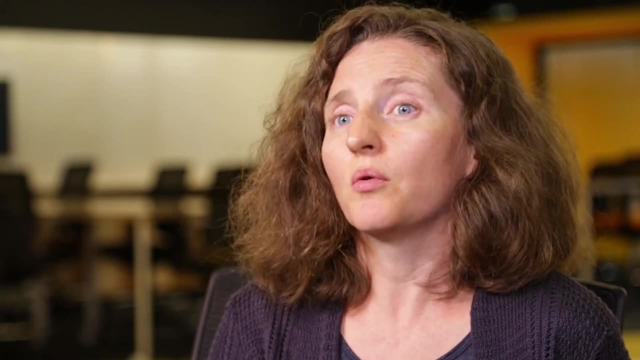 in an area that you don't know that much about but sounds kind of interesting from a student's point of view, From the course description. don't narrow yourself down, so get exposed to other stuff that you don't really know that well and you might find this really exciting. 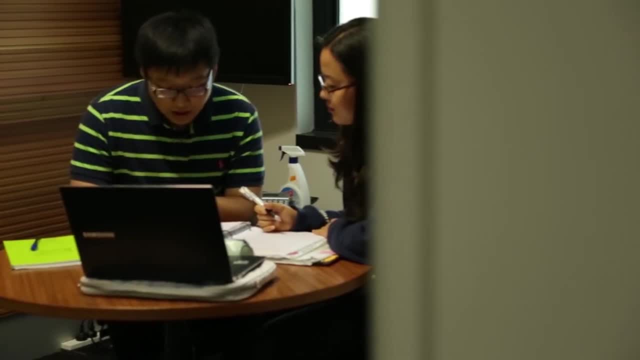 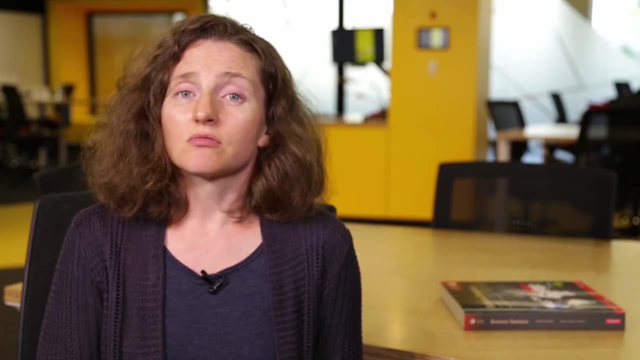 I guess I wish I knew about past classes, which is basically where two older students help guide you through the course in a really practical and easy to understand manner, which really would have helped me understand the difficult concepts that STATS is all about. So we have a great support system in place in this course, which consists of not only 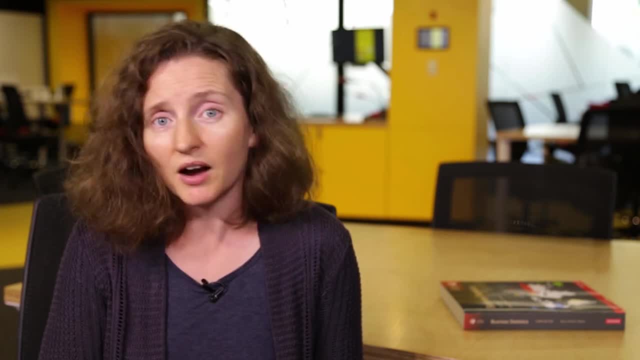 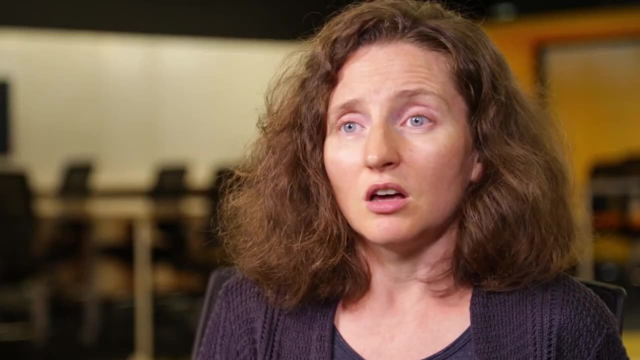 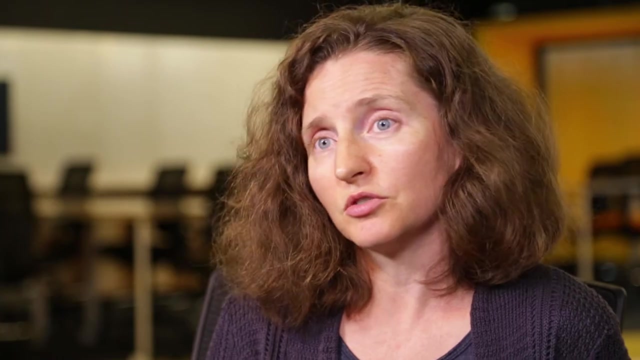 the normal lectures and tutorial workshops and consultation hours, of course, where I'm available and at your beck and call, no appointment necessary, people just drop in. but also a great online learning environment with the opportunity to ask questions and have them answered by either myself or other teaching staff or other students, If you don't come. 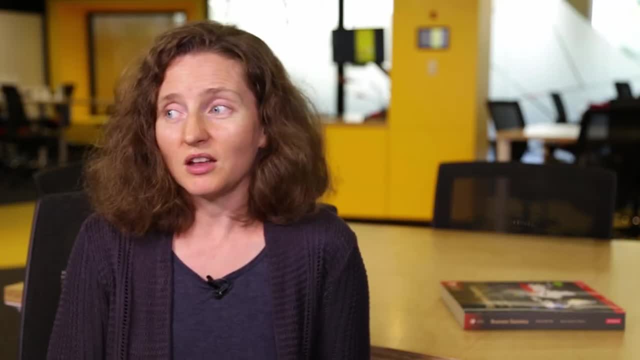 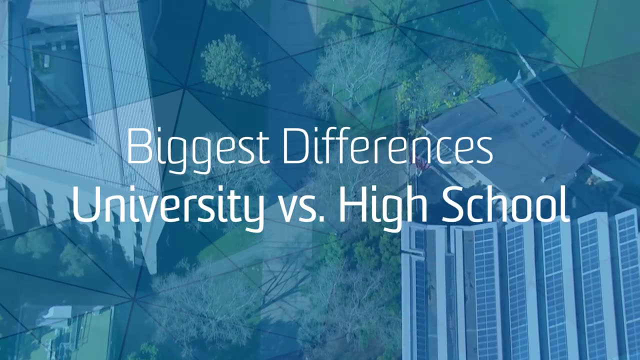 to office hours. you don't get to use that, so I hope that this video creates a lot of demand for office hours. I hope I'm really busy in my office hours this semester. So in this course we have the opportunity to use the new flipped classroom spaces. We